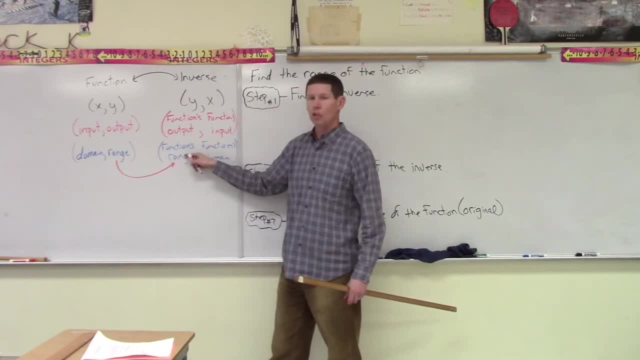 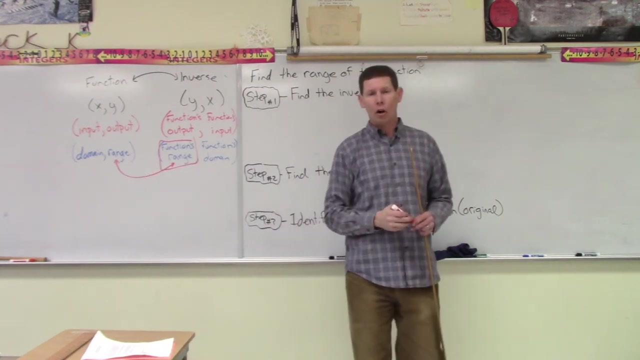 of our original function becomes the domain of the inverse function. So these values here, which would be the domain of our inverse, is the same as the range of our original function. That's going to be the key. So let's do an example. Let's do an example. 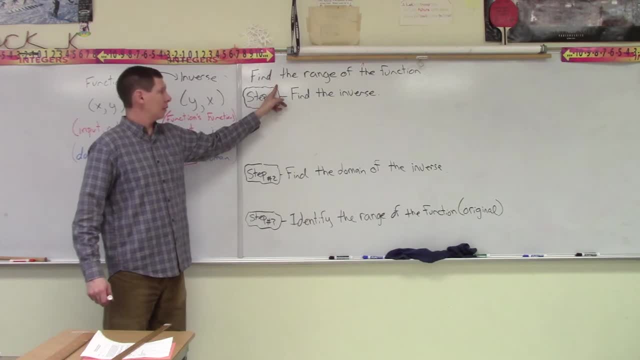 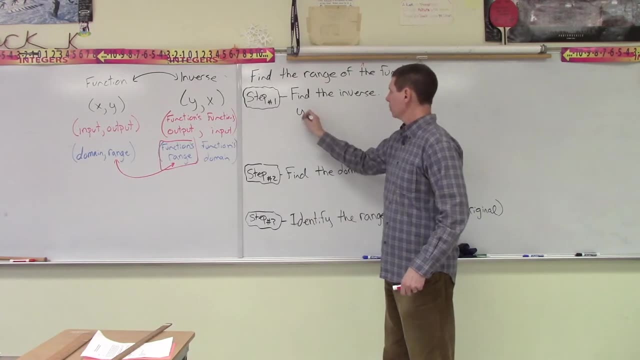 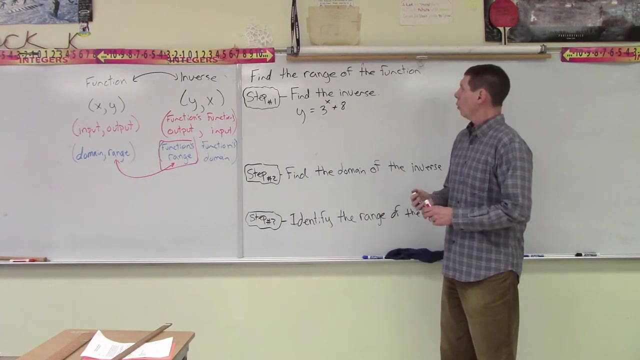 All right, Find the range of the function. Okay. Well, I suppose we should put a function there first. Let the function be: y equals 3 to the x plus 8.. So when we first have, the first step would be to find the inverse of this. Now, again finding the inverse. 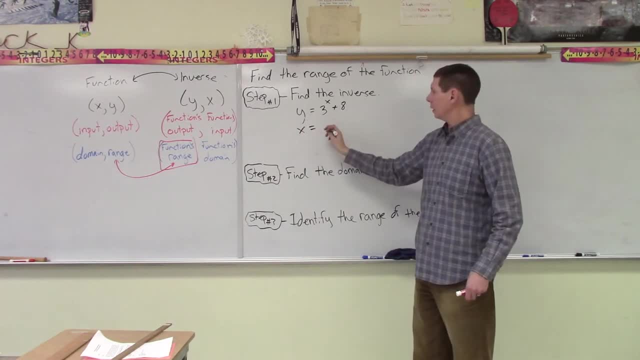 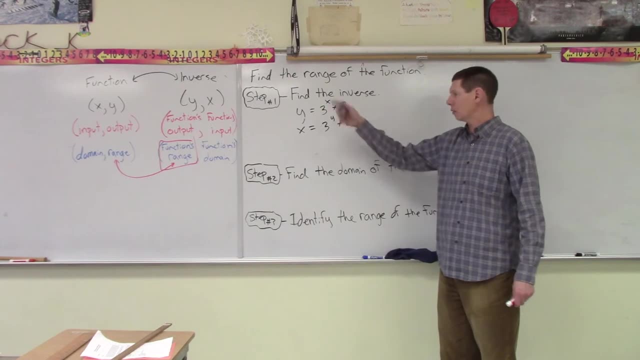 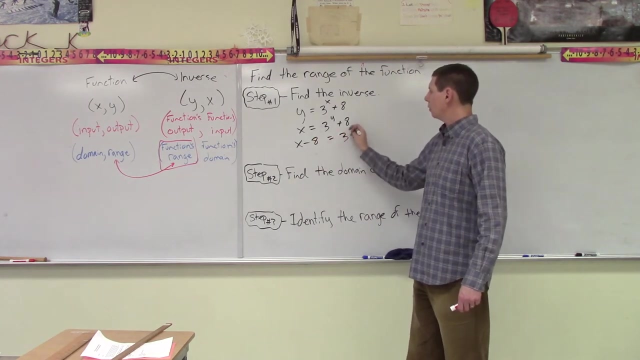 we'd be replacing y with x, okay, and x with y, Y with x, x with y, blah, blah blah. Now we could subtract 8 from both sides, so we get x minus 8 equals 3y, and this is a situation. 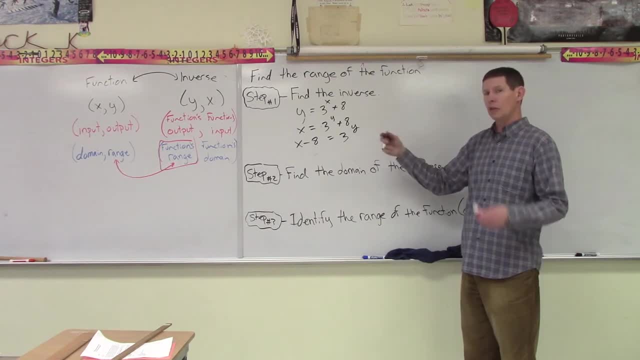 where we have an exponential equation or our variables tucked into the exponent which we need to get rid of. So our inverse of our exponential equation is going to be x minus 8.. Particularly that, for instance, the value of the exponential is using a logarithm. 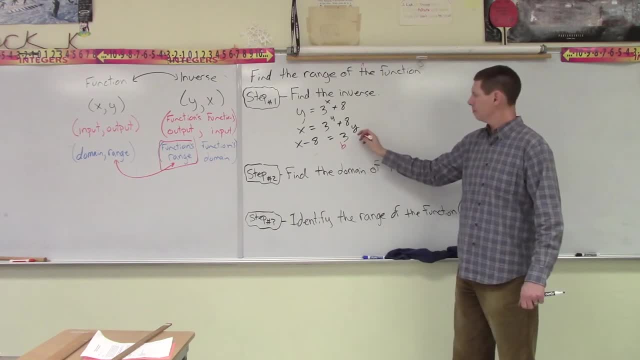 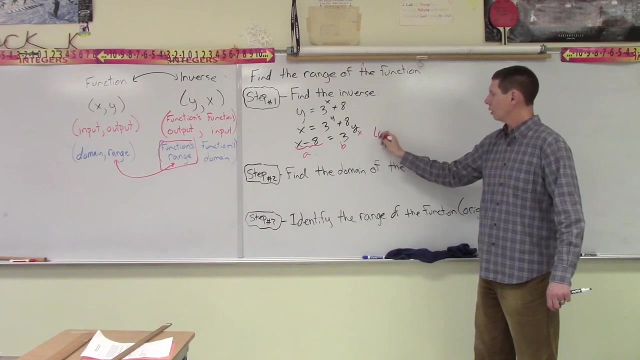 So if we take this as our b-value, our base, the y represents the x-value and the a-value is represented by x minus 8, we can take those three items, twist them into logarithmic form, so the log of our, with base-3, with the x minus 8 tucked behind it, that's going to. 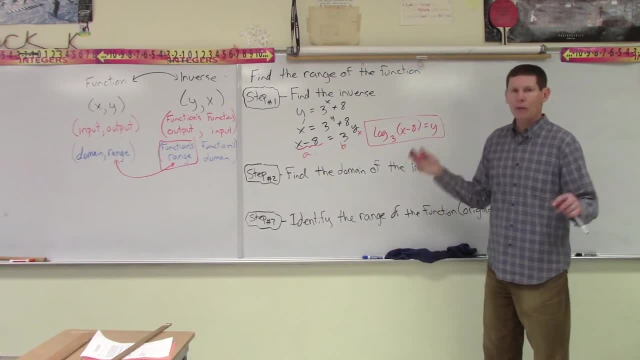 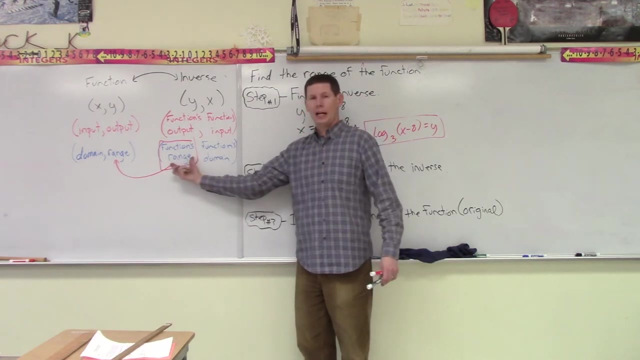 is equal to y. So that would be step 1, is finding the inverse relation. Step 2, we need to find the domain of this inverse. This is the key ingredient, because if we can find the domain of the inverse, in other words, all the values we can use as x coordinates, 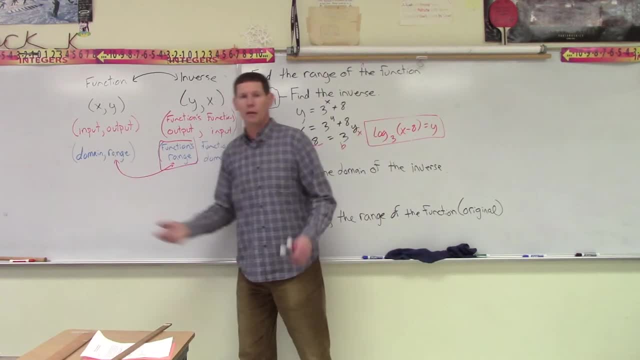 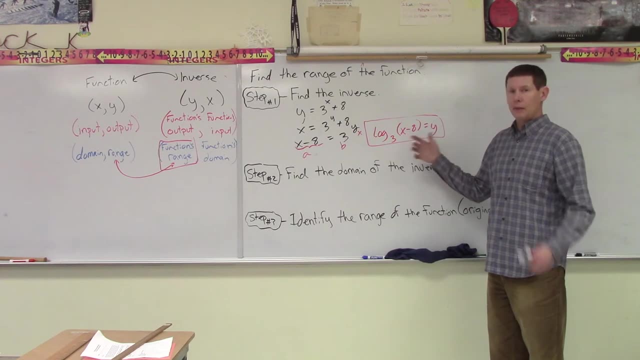 in our inverse that will be the same thing of the range of our original function. So let's think about how we find the domain. Again, we have to consider all operations. We say: can we subtract 8 from all numbers? Check the box, yes, we can. Are we allowed? 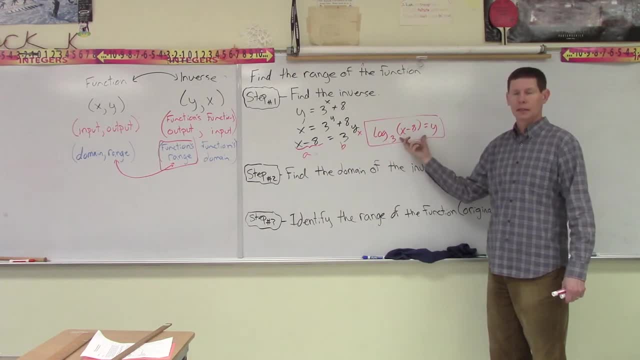 to take the logarithm of all types of numbers. No, We need to have positive numbers inside the logarithm. So to find the domain, there is a restriction, The restriction being whatever is behind the logarithm must be positive. So we have to write that: inequality of what's behind. 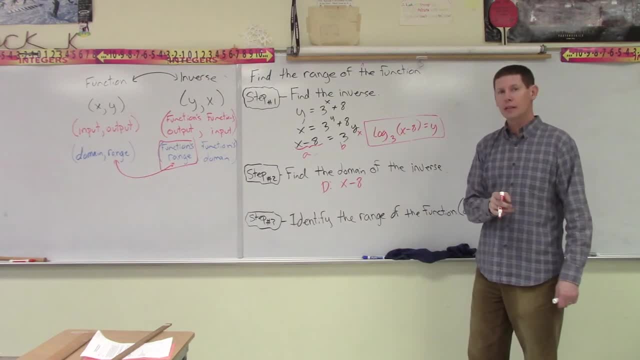 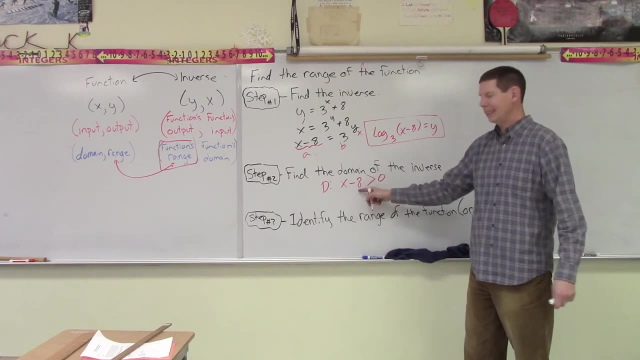 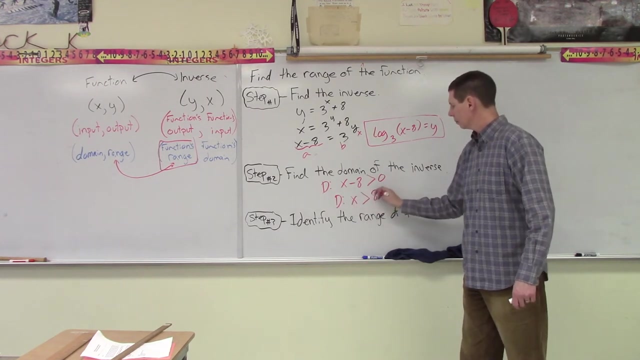 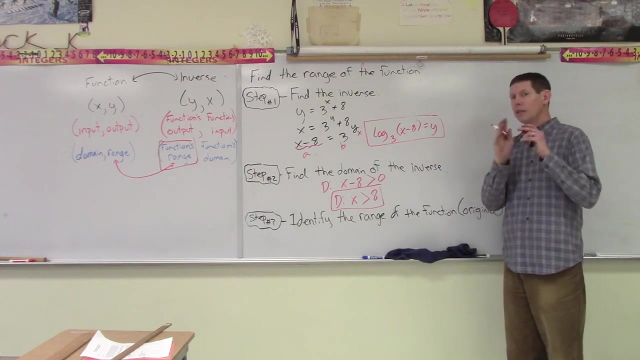 the logarithm, which is the x minus 8, and we have to make sure that is greater than 0.. So, in other words, let's not leave it like this. Let's add the 8 to both sides, And that would tell us the domain for our inverse relation, All the values that we are. 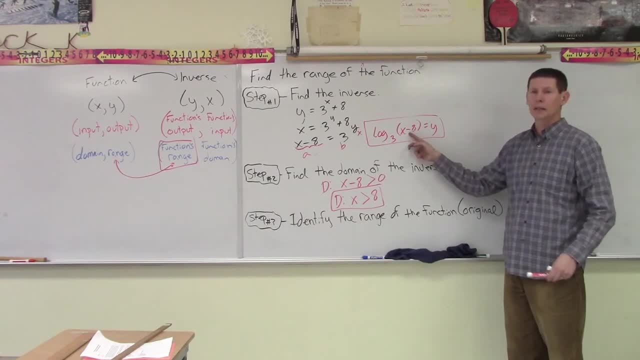 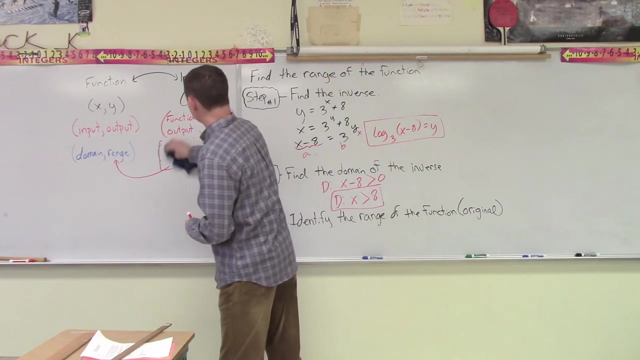 legally, mathematically allowed to put in. that makes this give us a result that's a real number, would be all numbers greater than 8.. Let's think of this in this setting. Okay, what we just figured out, okay, is that in 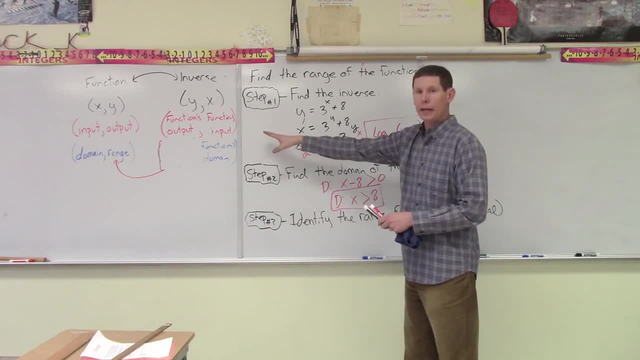 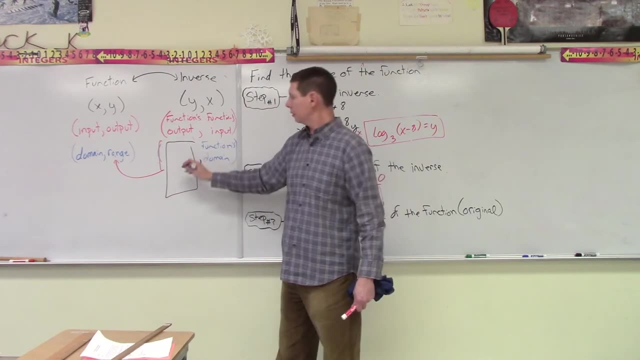 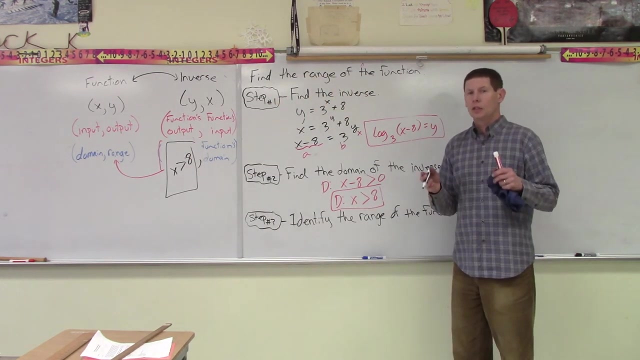 this ordered pair that represents our range. we just figured out. whatever we put in, the first number of the ordered pairs has to be all numbers bigger than eight. So if we understand what inverse relations are and the relationships between the input and output values, 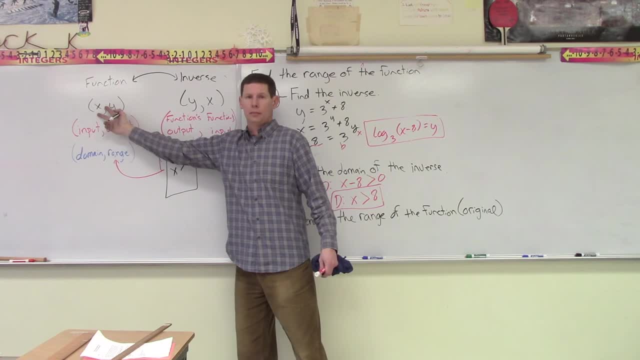 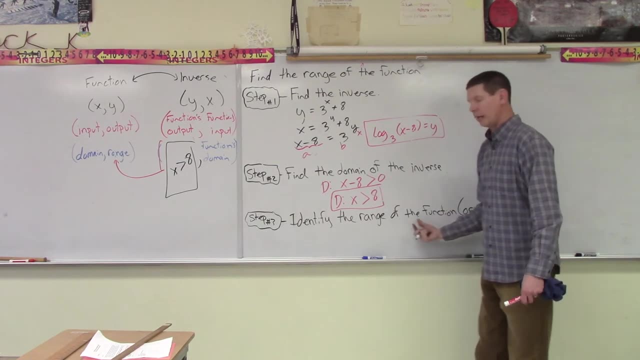 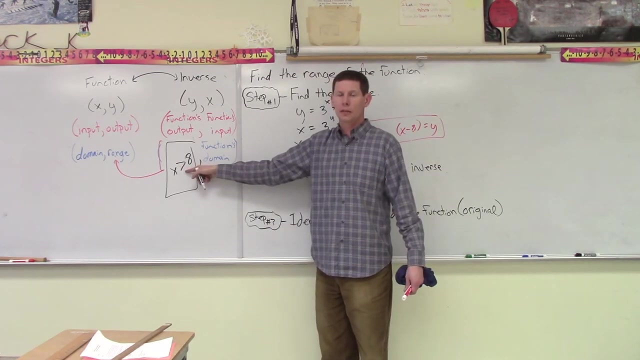 the x and y values between the original function and its inverse. we actually know step three. We want to identify the range of the original function or the function. we've already done. okay, It's this domain. it's the domain of the inverse. 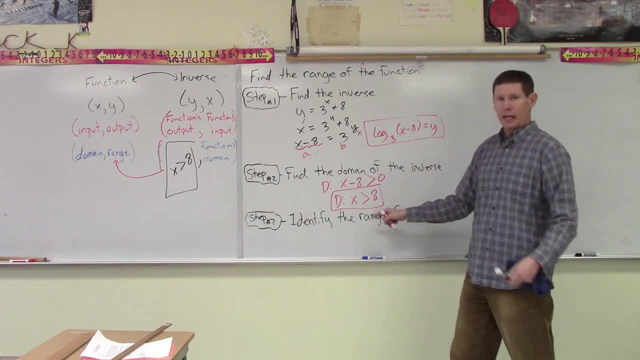 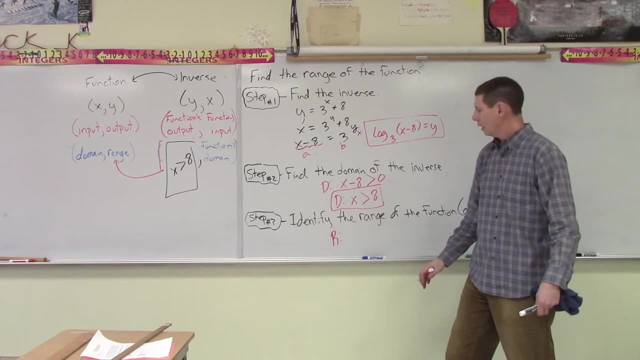 So let's just be careful on how we write it When we actually get to answering the questions. the original question: find the range. we would say our range. I'm gonna put R there instead of D is gonna be, and now our range deals. 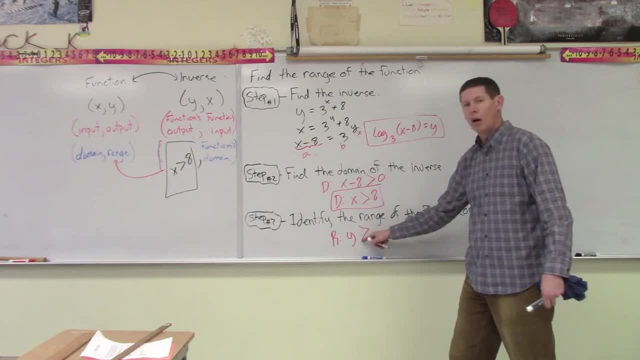 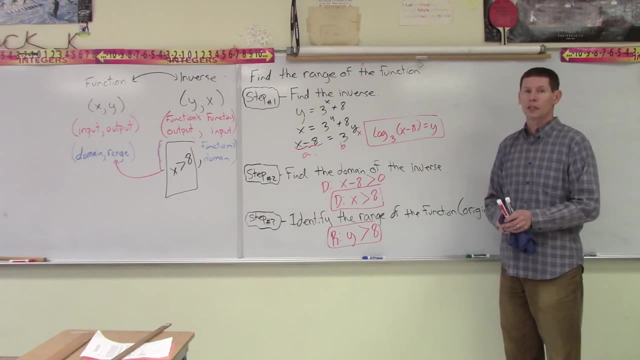 with the y-axis, Y-coordinates, so all y values greater than eight. okay, So that's how you find the range. three easy steps: Find the inverse of the given function, find the domain of that inverse and rewrite that domain as a range.